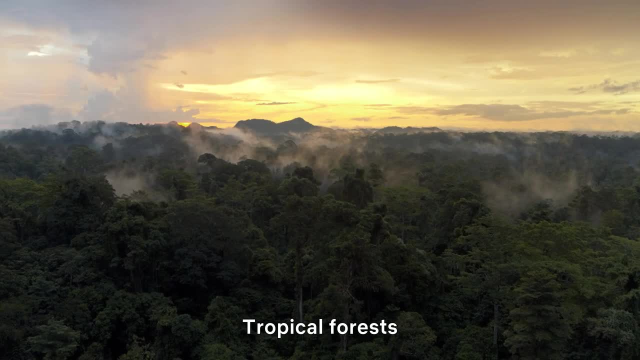 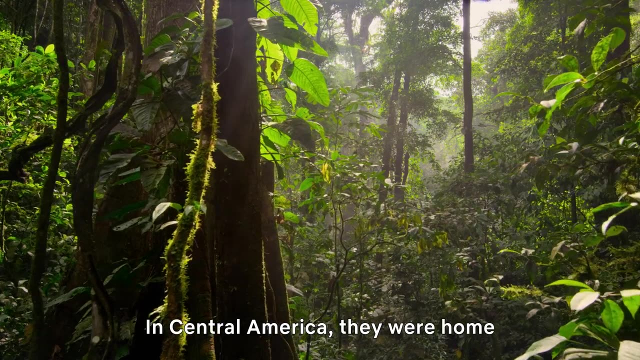 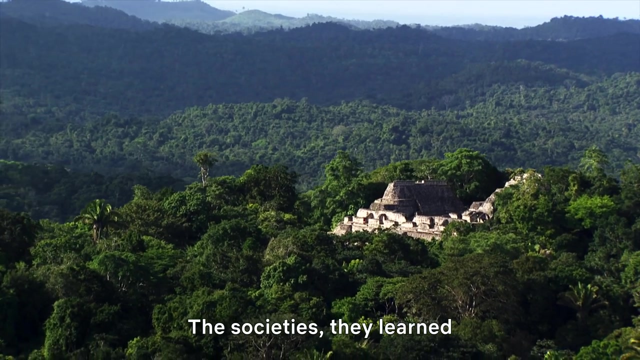 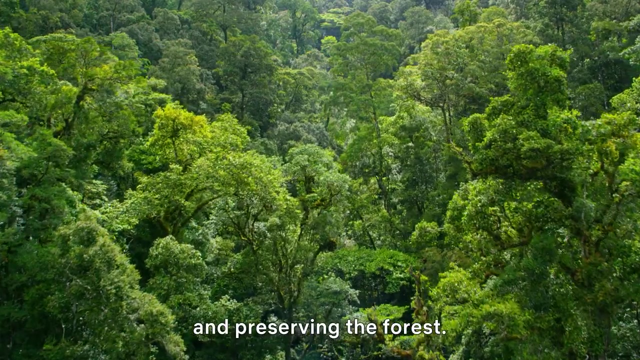 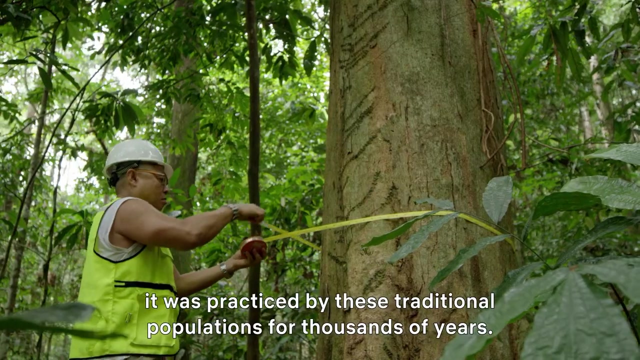 Tropical forests exist for more than 100 million years In Central America. they were home to at least 25 million people, These societies, they learn how to live with the forest, out of the forest and preserving the forest- The idea of sustainability that we have today. it was practiced by these traditional populations for thousands of years. 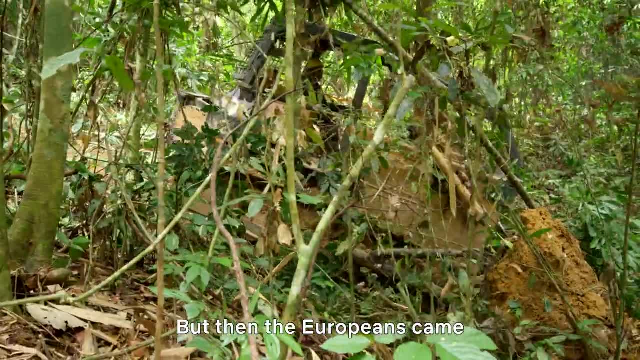 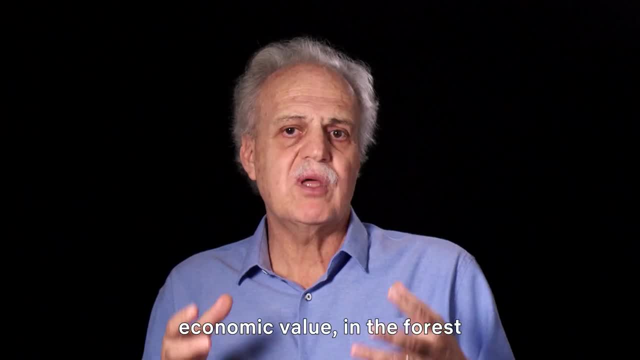 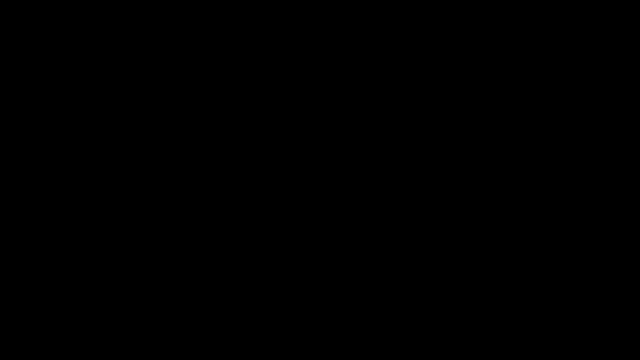 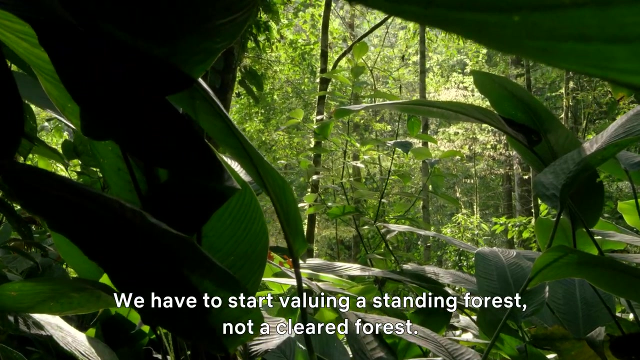 But then the Europeans came and they started cutting down the forest. They were not able to see value, economic value, in the forest And unfortunately, this is still the prevailing view even today. We have to start valuing a standing forest, not a clear forest. 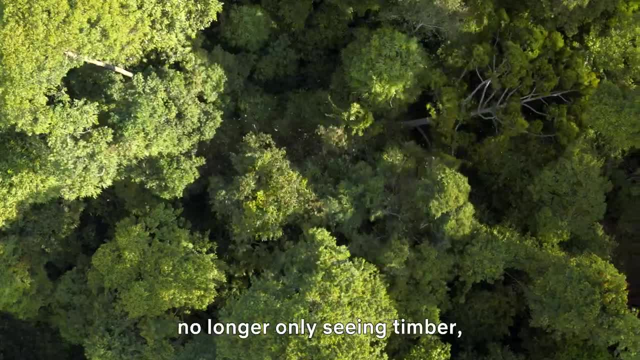 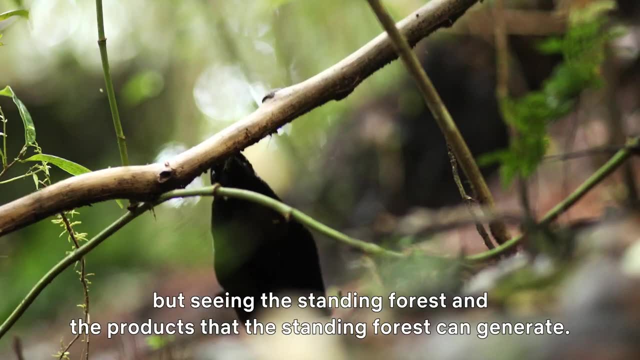 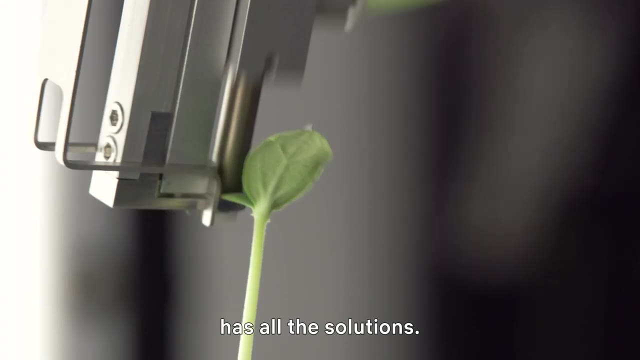 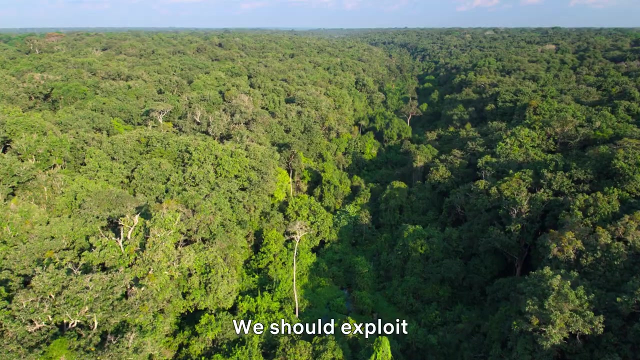 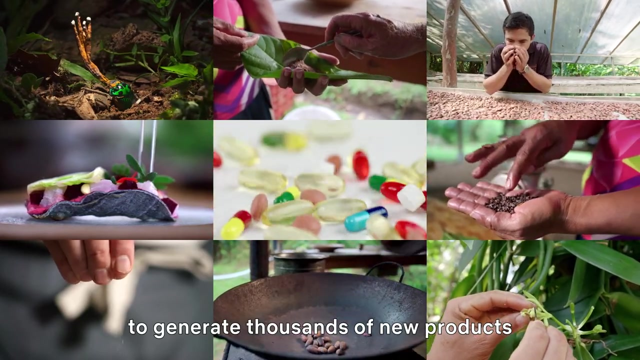 No longer cutting down the trees, no longer only seeing timber, but seeing the standing forest and the products that the standing forest can generate. This is possible. Applied science, modern agronomy has all the solutions. We should exploit standing forest bioeconomy to generate thousands of new products with the standing forest. 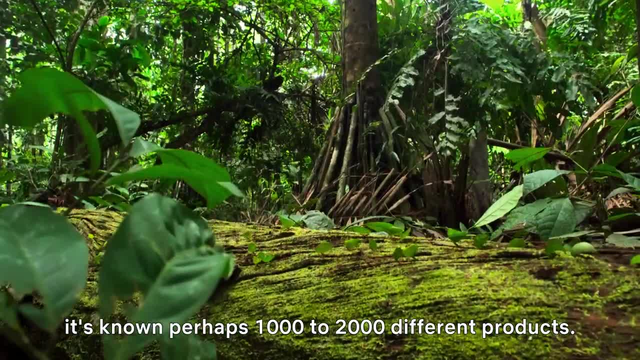 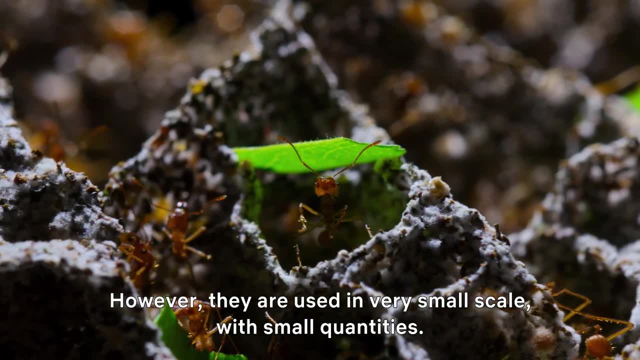 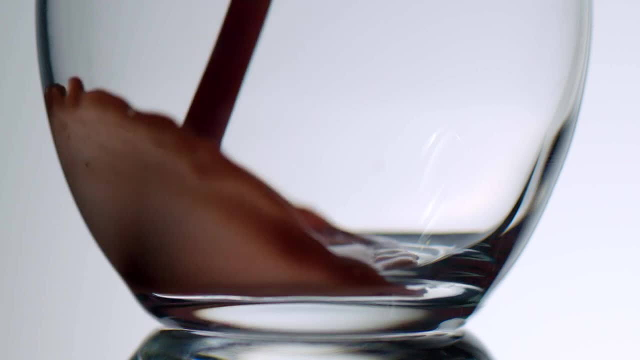 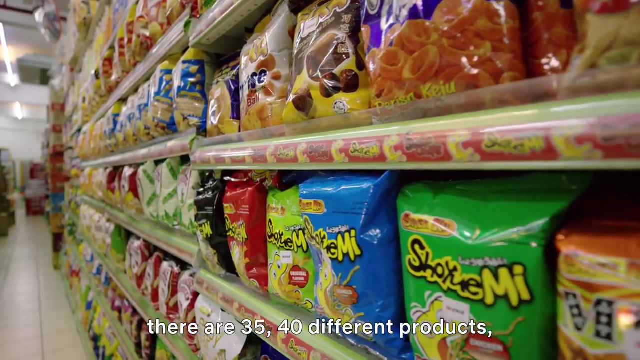 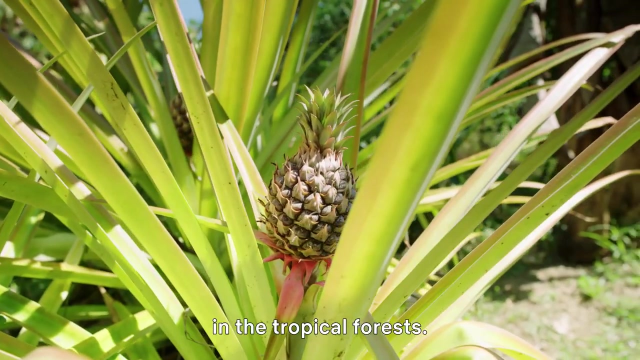 In the Amazon in particular, it's known perhaps 1,000 to 2,000 different products. However, they are used in very small scale with small quantities. But there is one exception. It's called acai Today, acai berry. in the global markets there are 35, 40 different products, produced mostly in agroforestry systems in the tropical forests. 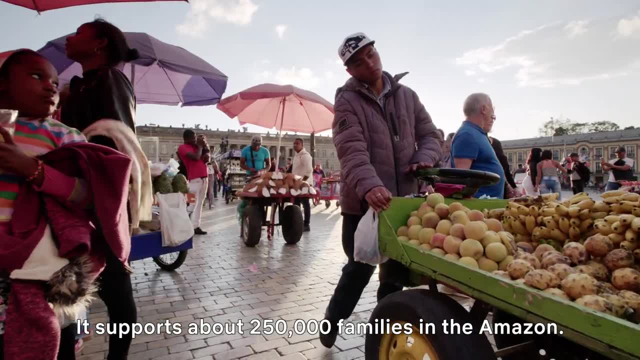 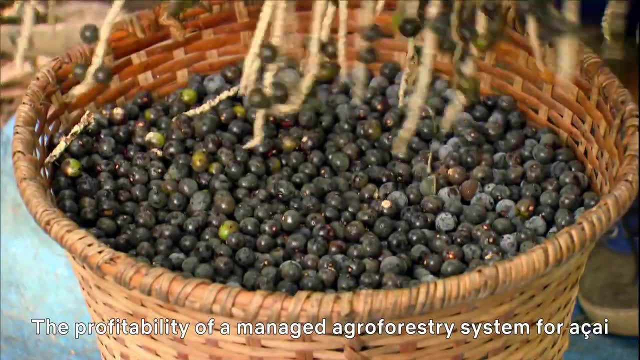 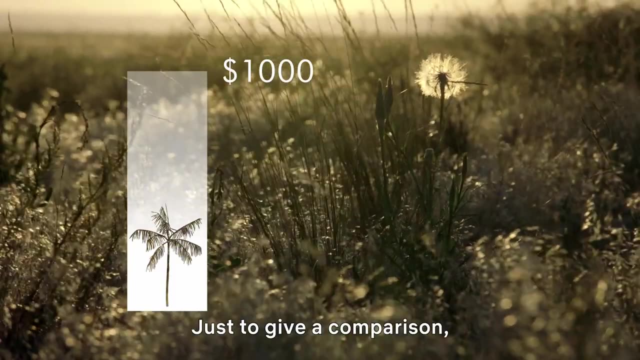 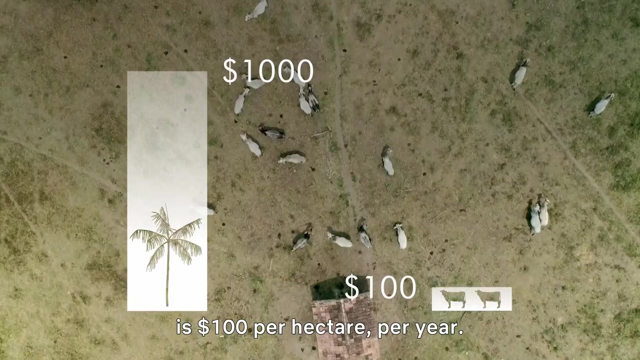 It supports about 250,000 families in the Amazon. The profitability of a managed agroforestry system for acai is about $1,000 per year per hectare. Just to give a comparison, a very well-managed cattle ranch in the Amazon is $100 per hectare per year.